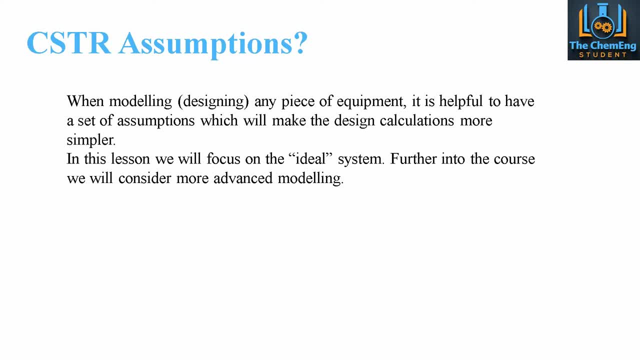 and some examples for these kind of systems as well. So be sure to go and check that out via our website. So the assumptions that we're going to make here for the ideal CSTR is that we have steady state conditions. therefore we have no accumulation within the system. 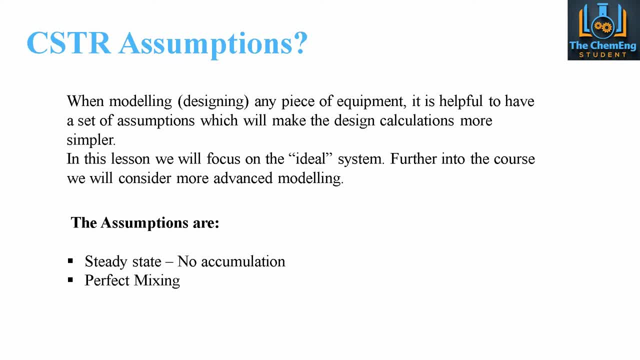 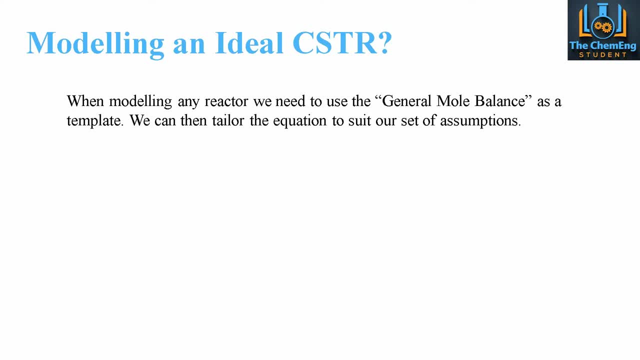 and that we have perfect mixing throughout. Now, when we model any of these reactors, we use what's known as the general mole balance, And this is a template in which we can tailor to suit our set of assumptions. So what we have here is we see that the amount of A that is introduced per unit time must be equal. 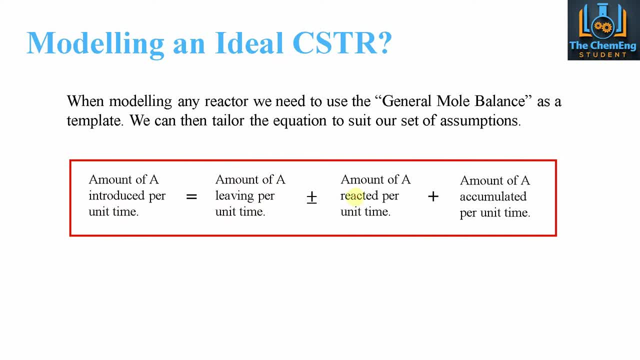 to the amount of A that leaves per unit time, plus or minus the amount of A that reacts per unit time, plus the amount that is accumulated of A per unit time. Now we can rewrite this in terms of nomenclature, whereby we have F, so F naught and F. these are the flow rates. 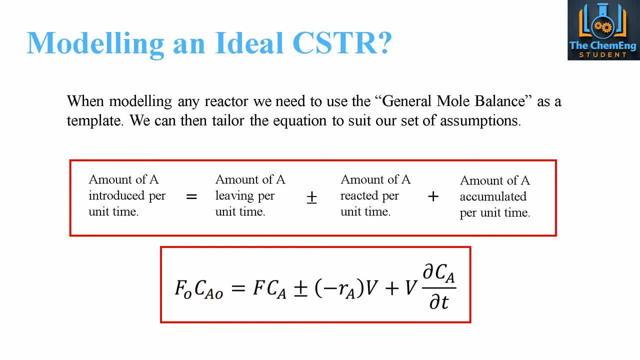 C A naught is for the initial concentration of A. C A is the final concentration of A. Now we have plus or minus here, because depending on whether we are reacting A or producing A, we'll determine whether or not this value is positive or negative. 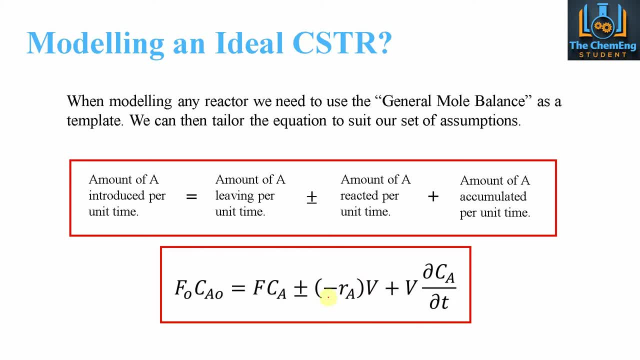 And then for the actual reaction itself, what we have is the rate expression, so minus R A multiplied by the volume of the system plus, and then the accumulation term is the volume multiplied by the partial differential of the concentration with respect to time. 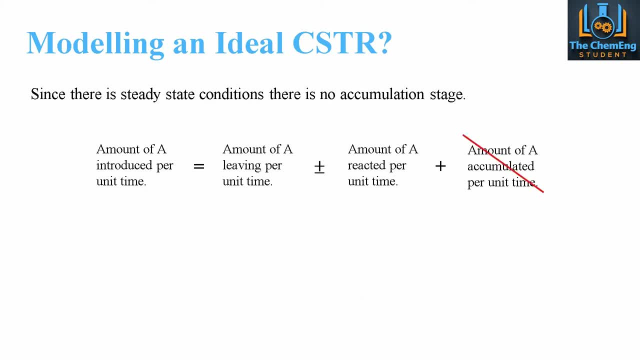 Now, since we have steady state conditions, we can neglect the accumulation term, which means our equation would rewrite as the following: whereby we can cancel out this term here. So what we're left with is F naught C A. naught equals F C A plus or minus. 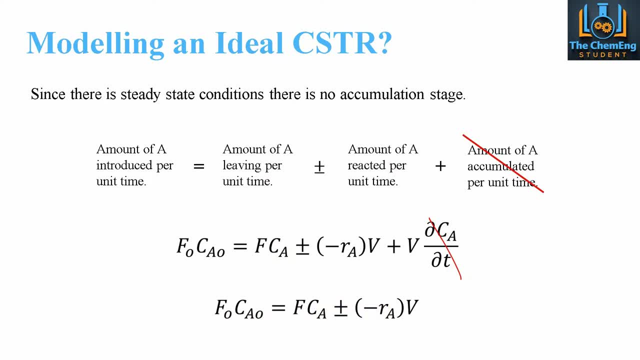 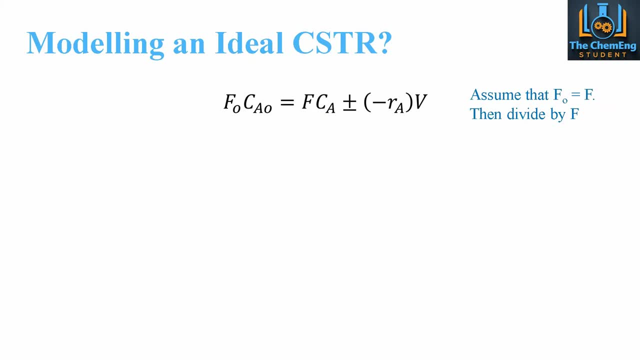 minus R A multiplied by the volume. Now, the other set of assumptions that we made was that we have steady state conditions, so, and we also have perfect mixing. so what we can then say is that F naught must be equal to F.